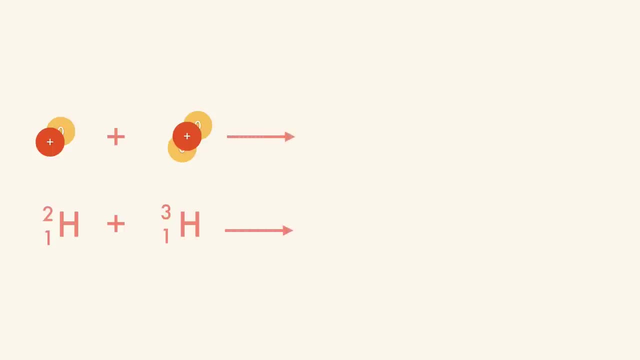 When they collide under high-temperature conditions, they form a helium atom with two protons and two neutrons. They release a neutron written with the lowercase n for the symbol and they release a huge amount of energy. Now it would be amazing if we could harness this massive release of energy to feed our sun. 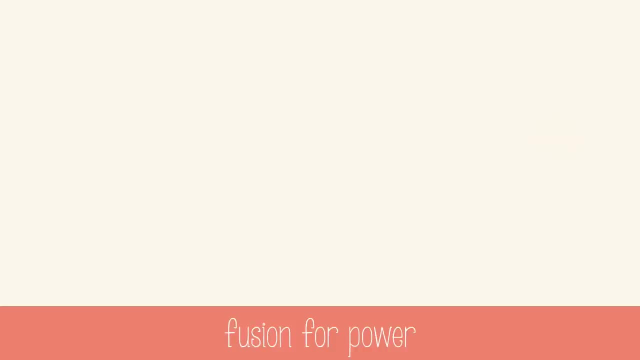 That would be our need for electrical energy. but we run into two problems with fusion. Fusion requires temperatures that are very high and very difficult to attain, and the reaction itself is nearly impossible to control. To get the high temperatures to start the reaction we need something like a nuclear bomb, and once that's going, good luck trying to control it. 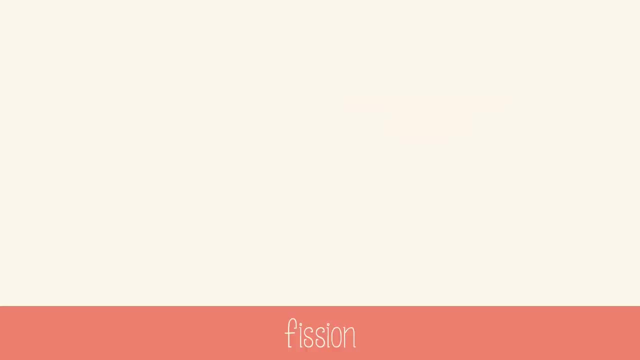 Fusion is in a small part the opposite of fusion. It's the splitting of a nucleus into smaller fragments by the release of neutrons and lots of energy. But nuclear fission will only happen when neutrons hit one of two fissionable isotopes. 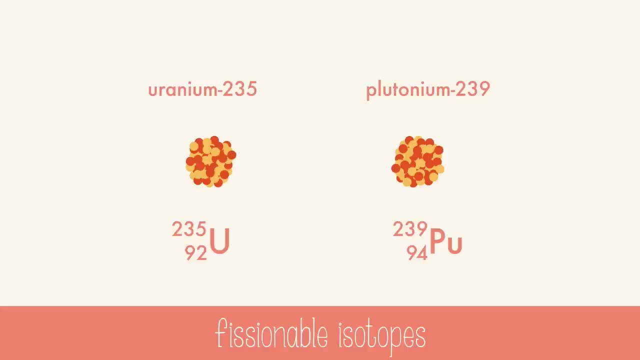 uranium-235 or plutonium-239.. First, a neutron hits uranium-235,, which makes it so unstable. it breaks into two smaller parts and also releases three neutrons. If these neutrons hit other uranium-235 atoms, it can start a chain reaction. 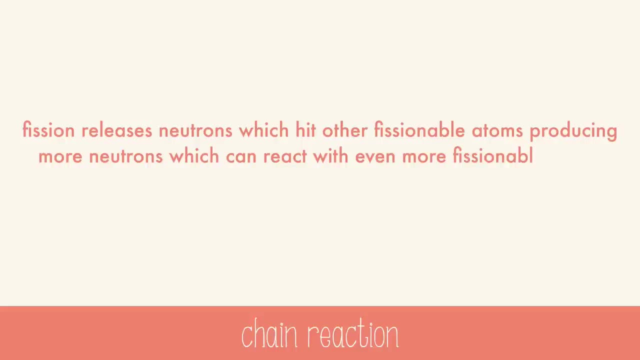 A chain reaction is where fission releases neutrons which hit other fissionable atoms, producing more neutrons which can react with even more fissionable atoms, and so on and so forth. We can harness the energy released from fission much more easily than harnessing fusion's energy. 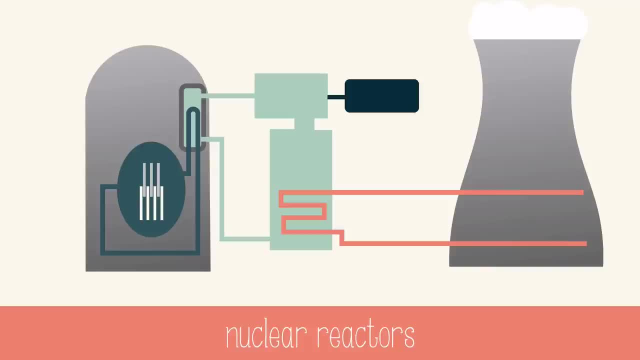 Nuclear reactors are the heart and soul of nuclear power plants. We use controlled fission in fuel rods that are cooled by a coolant fluid, usually water. The heat from the core is used to generate steam, which will drive a turbine that creates electricity and a generator. 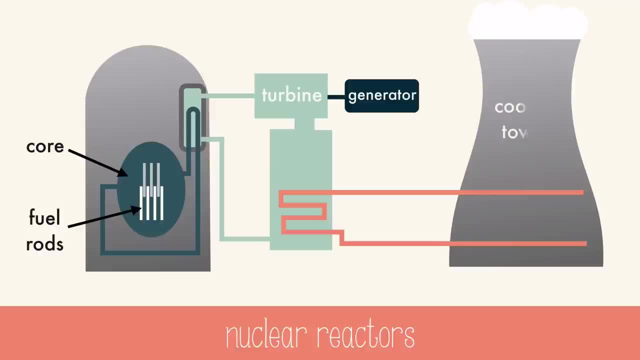 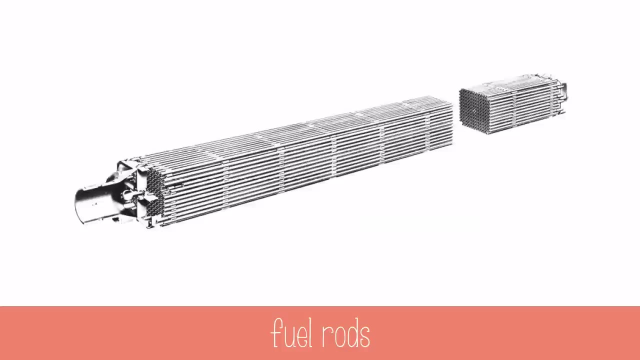 The large towers that you may be used to seeing are actually just for cooling down and condensing the water so that it can be reused in the system. There's no radioactive material in those cooling towers, just steam. The fuel rods are made of a metal which contains uranium-235 or plutonium-239..